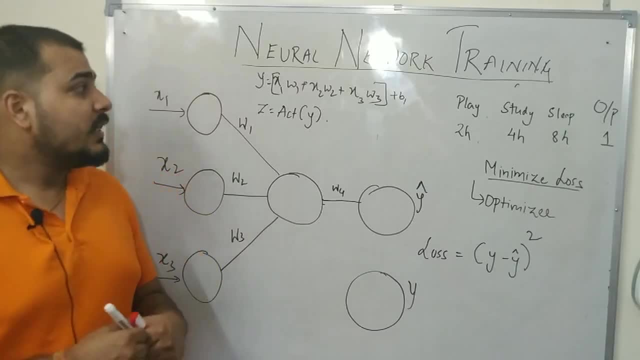 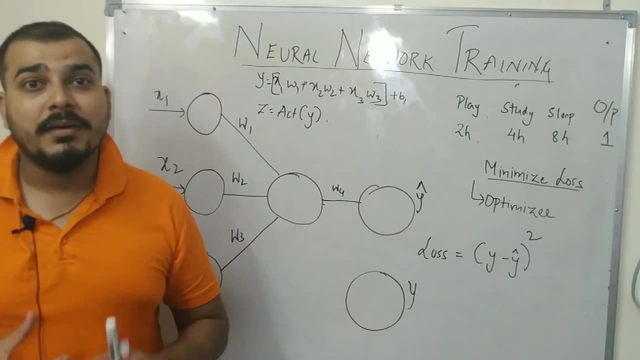 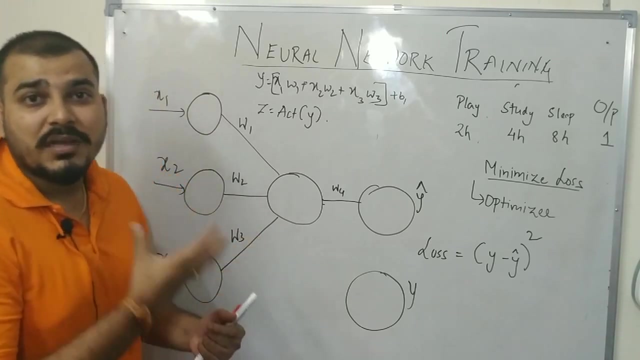 Hello all. my name is Krish Naik and welcome to my YouTube channel. We'll continue the session and today we are basically going to discuss about neural network training. How does neural network training happen? I'm also going to include you both forward propagation and backward propagation. I'm also going to introduce you some of the concepts like loss, function optimizer and all. So let us just understand. In our previous videos, I've already shown you what are the different architecture, what is the architecture of a normal neural network and what kind of activation functions basically gets applied. 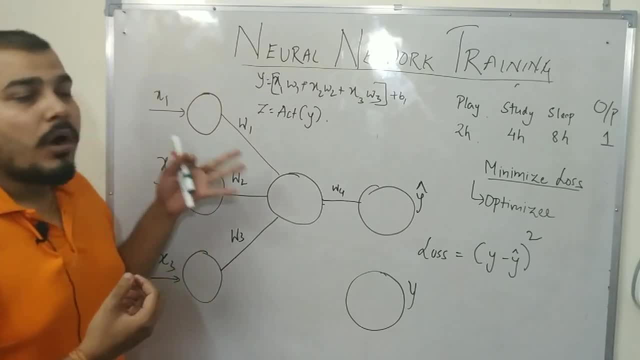 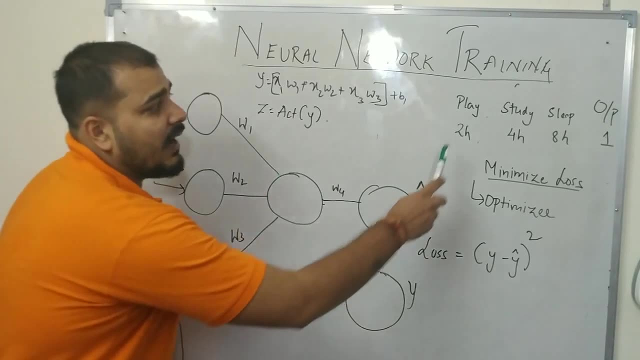 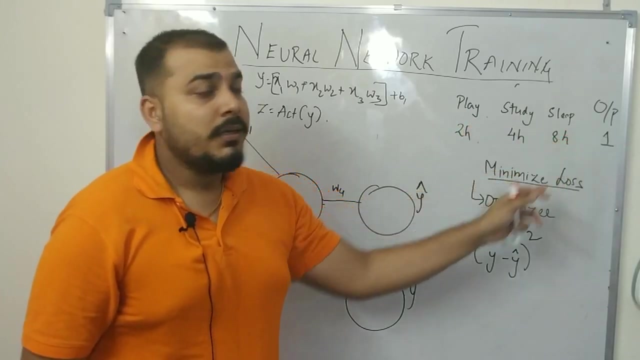 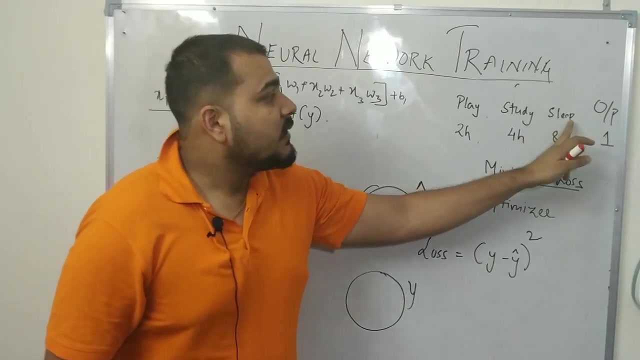 We discussed about sigmoid and relu, but let me just discuss how the training of this neural network happens in an artificial neural network. So to begin with, guys, let us consider I have a data set which looks something like this: Play, study, sleep. I have three features. which is like play, study, sleep. In the play it shows that a student plays for two hours and in study it shows that he studies for four hours. and in sleep he has a data set where he's sleeping for eight hours and the output is basically ones and zeros. 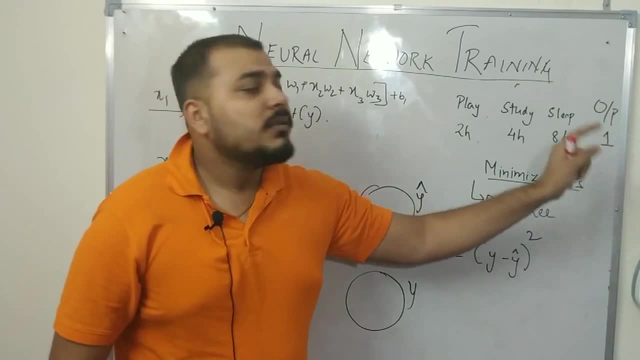 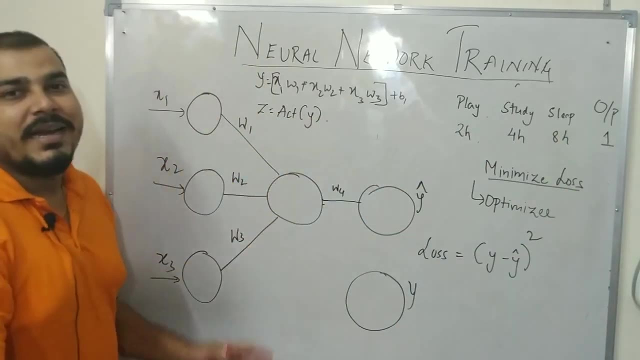 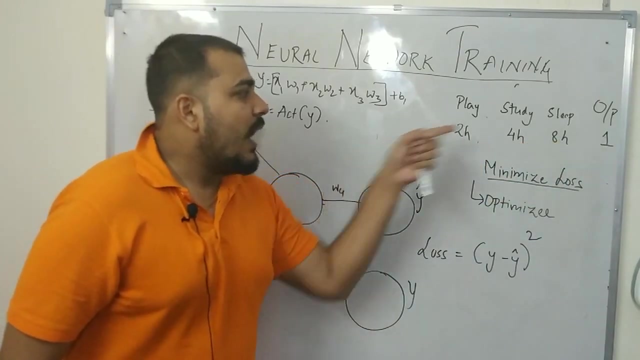 One basically indicate that the student will pass the exam. Zero basically indicates that student will fail the exam. Now let us just take this particular example and see how this particular data set, how this problem statement, will be getting trained in our neural network. So first I'll start with forward propagation. So you all know I have inputs x1,, x2, x3. This is my x1, this is my x2, this is my x3. So I'm just considering one record right now. All these input features will get passed to my hidden neural network. 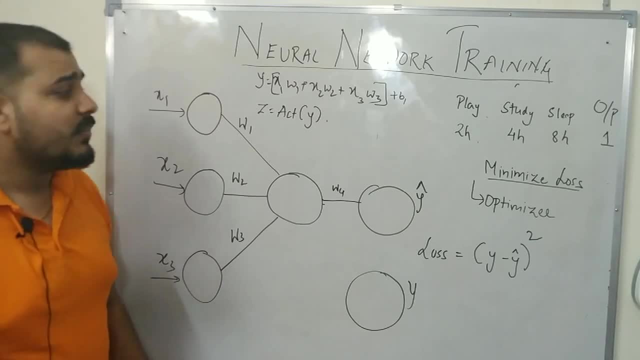 Okay, so I'm just considering one hidden neuron to just show you an example how this particular pre-processing, how this particular training will actually happen. So all these input features will go over here. So I have all my input features. that is going over here. After this input feature goes, what happens is that then we this two important steps happens. This two steps happen Once. first step is basically where we'll multiply the input features with the weights, The summation of all this input. 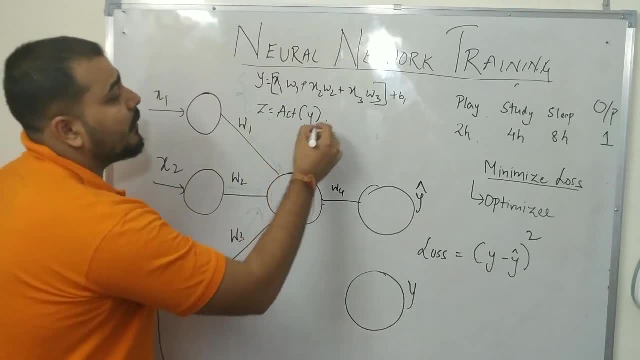 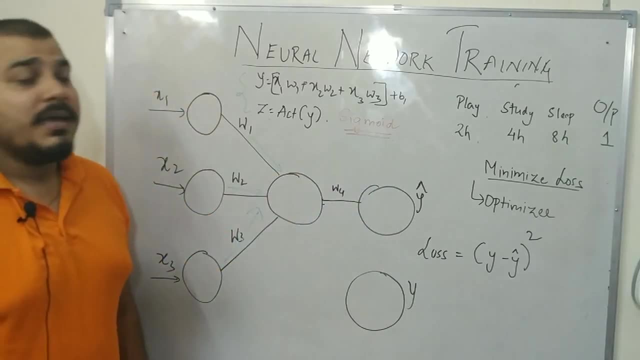 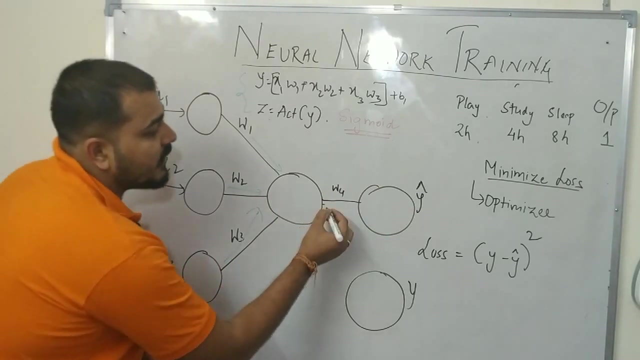 and the features will happen, plus the bias, and then an activation function is applied. Activation function may be sigmoid, It may be sigmoid. Okay, sigmoid activation function may apply. and you know that sigmoid activation function transforms your value between 0 to 1.. Okay, so here, once it is getting transformed, then what will happen? next input, next next step, is that it will go and pass to the output layer. Here also, some weights are basically assigned, So this will get passed to the output layer After it gets passed to the output layer. 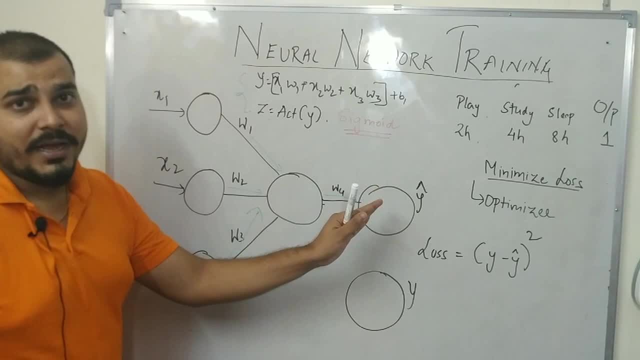 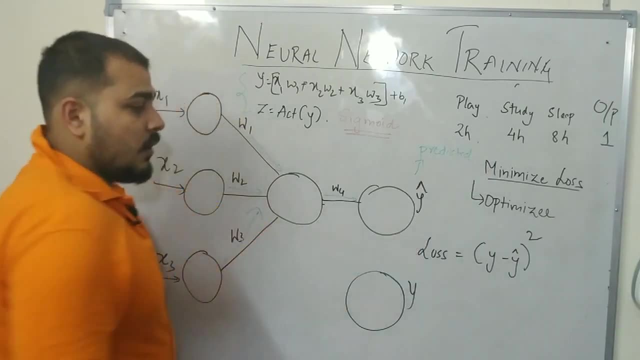 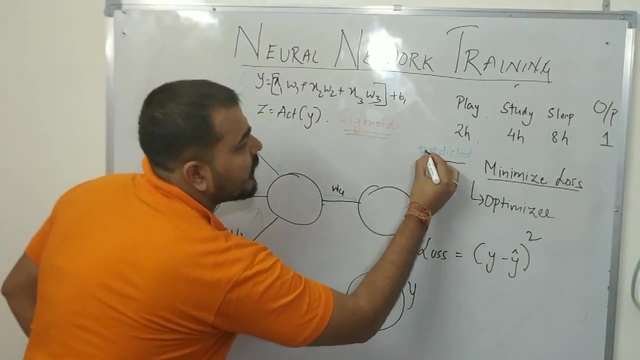 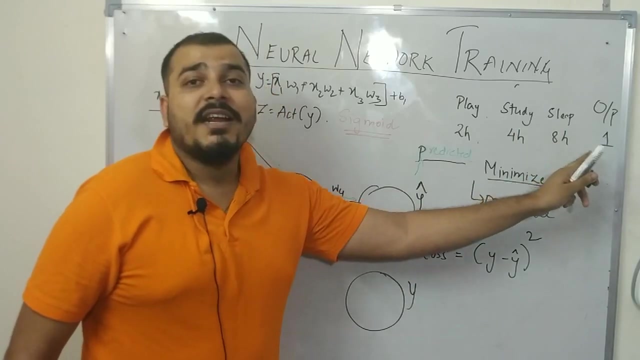 this particular value, y hat. this layer is basically the output layer. Now y hat will be my predicted output. So this will be my predicted output. Okay, I'm just sorry for the lighter link. So this will basically be my predicted output. Okay, now I already know that in my training data set the output for this kind of data is 1.. Now suppose my y hat is basically predicted as 0 over here. 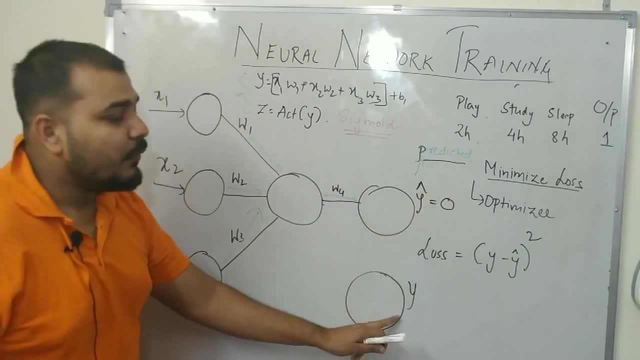 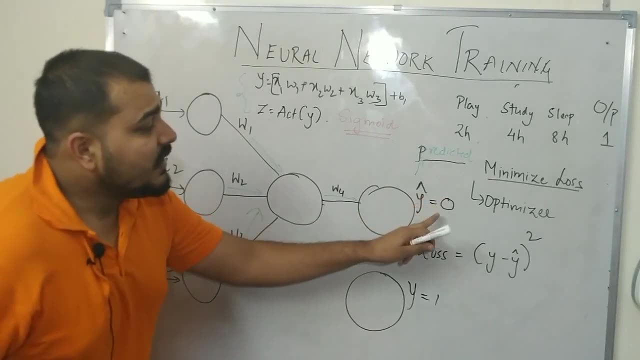 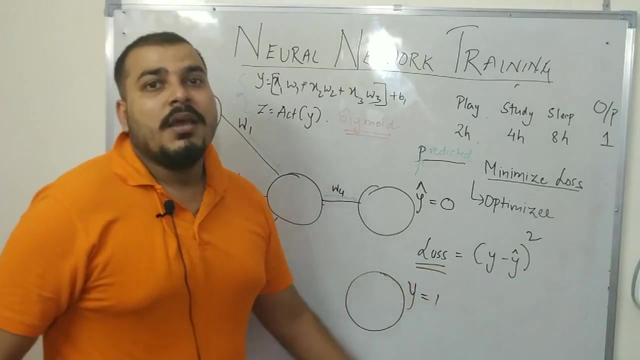 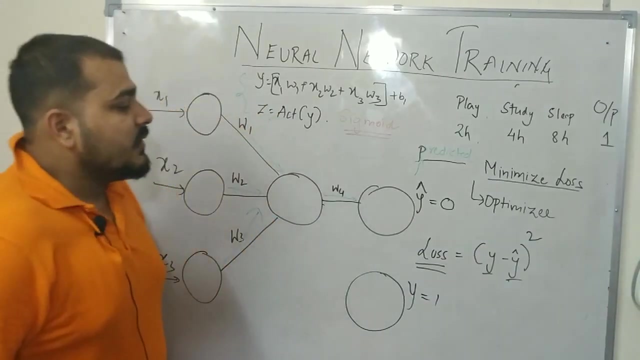 But we know that we need to compare this, whether this y hat and y are almost same. So currently, for this record, the my y value is 1.. So what we do is that we try to see this differences, and that difference can be found out by a loss function. And this is the formula of a loss function, where I'm actually subtracting my actual value with my predicted value: whole square. The reason I'm doing the whole square is that sometimes this may become 0, this may become 1.. So whenever the negative value is coming, and if you do the square, 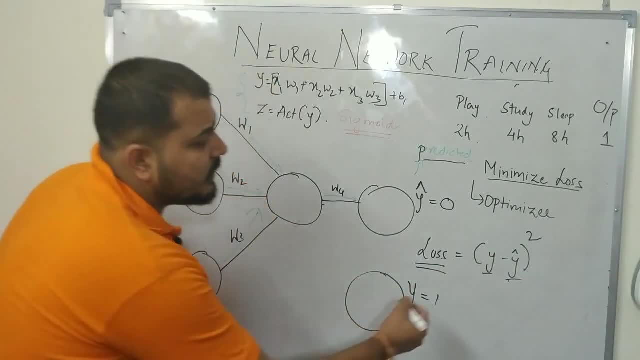 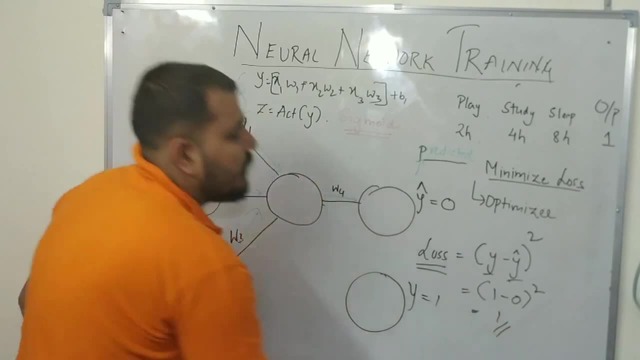 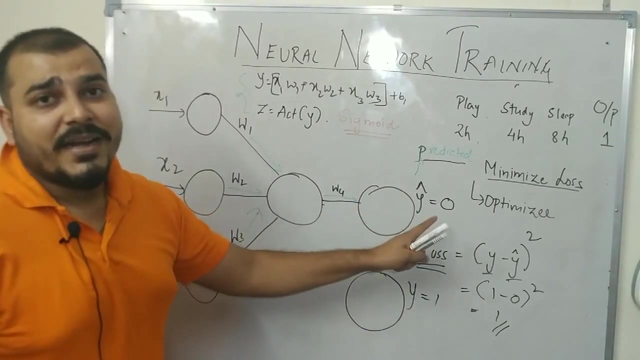 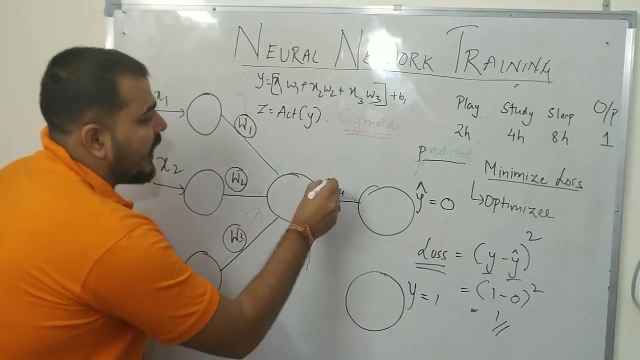 of that will become a positive value. Now, in this case, you will see that my y is basically 1, my y hat is 0. So this becomes 1.. Right Now, here you can see that the loss value is higher. Okay, it is 1.. And by the difference also, it is completely wrongly predicted, right? So we should try to adjust this weights. this weights adjusting must be done in such a way that for this particular record always, my predicted output should be 1.. So for 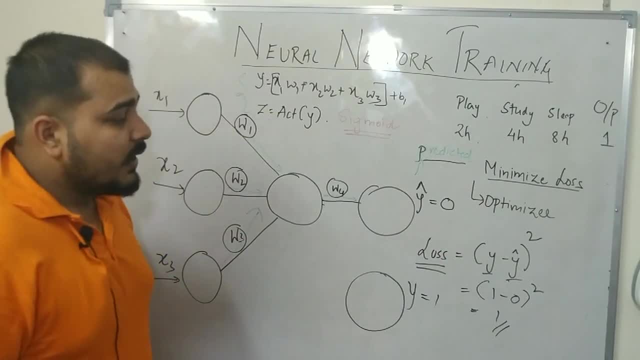 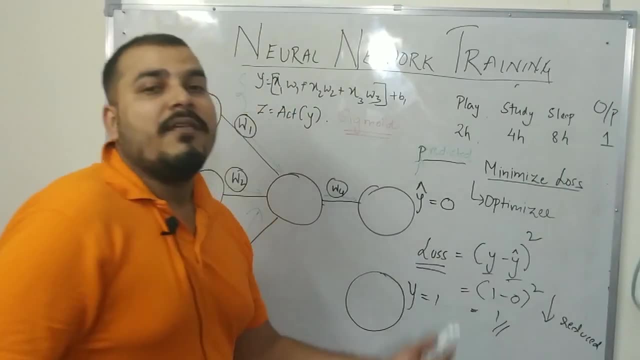 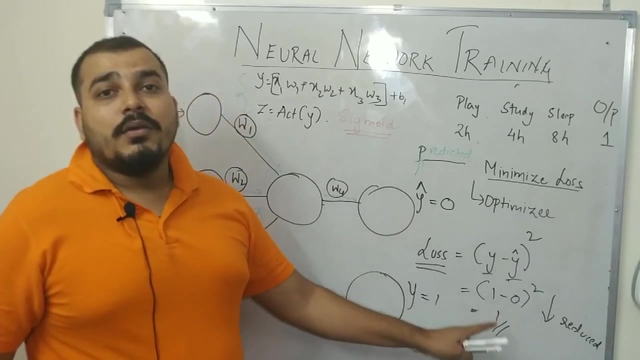 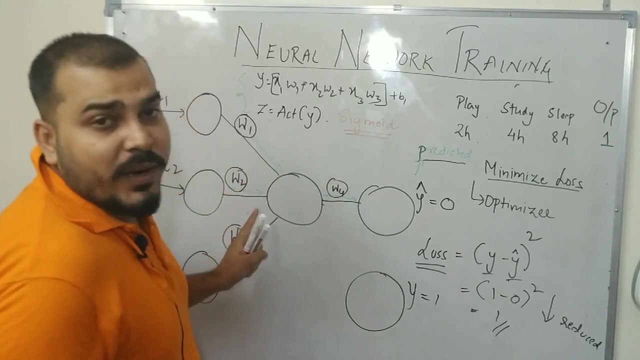 that what we do is that we define a loss function. Now, after defining a loss function, this loss value should be reduced. It should be reduced to a minimal value such that our y hat should match y. Now, in this scenario, you can see that my loss function is having the value as 1.. So, during the training phase, I should be updating this weights. Okay, I should be updating these weights in such a way that this loss value should be decreasing, decreasing, Okay. 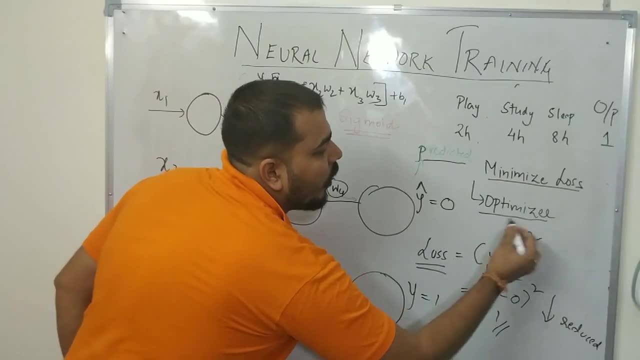 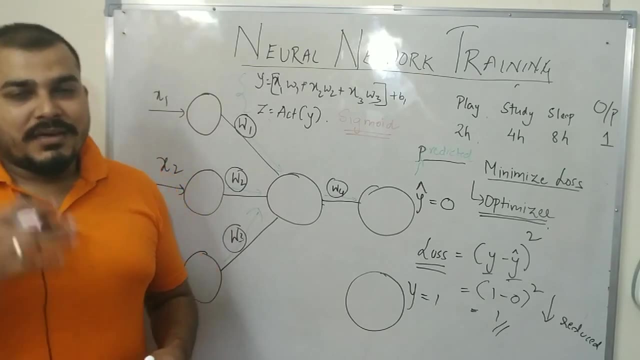 So how it can be done. It can basically be done by using an optimizer. Okay, there are a lot of optimizers that are basically used in deep learning. Some of the optimizers are gradient descent, stochastic gradient descent and many more. As we go ahead, we'll be discussing about this- all optimizers- in our future classes. But now, what will happen now? Now I've got my loss value over here, my optimizer will try to reduce this loss value. In order to reduce this loss value, we basically have to back up this loss value. So, in order to reduce this loss value, we basically have to back up this loss value. So, in order to reduce this loss value, we basically have to. 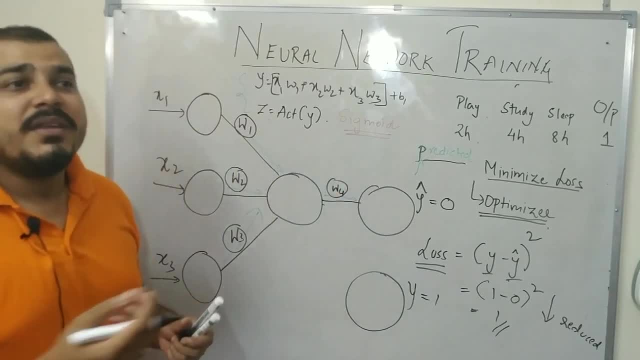 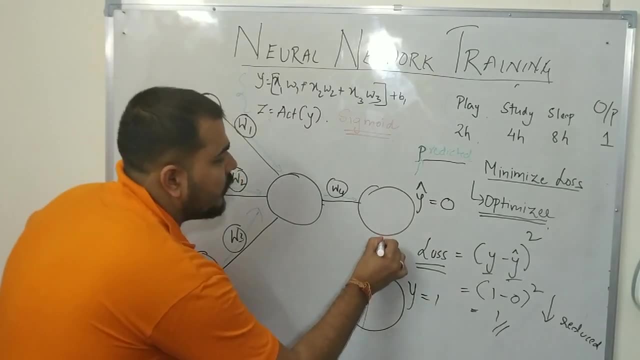 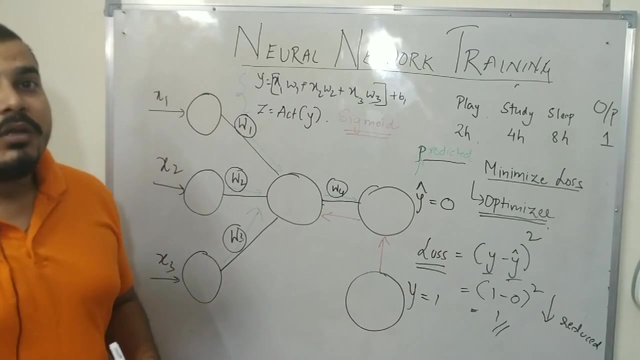 back propagate. now, When we do the back propagation, that basically means we have to update this weights Now to do the back propagation. what we do is that first of all I'll draw a line back. Okay, Now, during this back propagation, this weights will get updated. How the weights will get basically updated is that this weight- suppose my W4 new- has to be getting calculated right Because I have to update W4. Now this can be updated by taking the W4 weight. 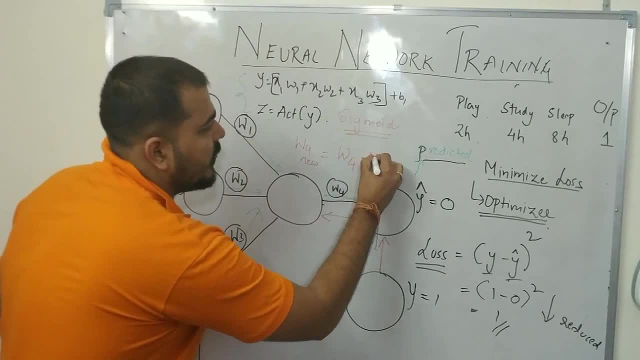 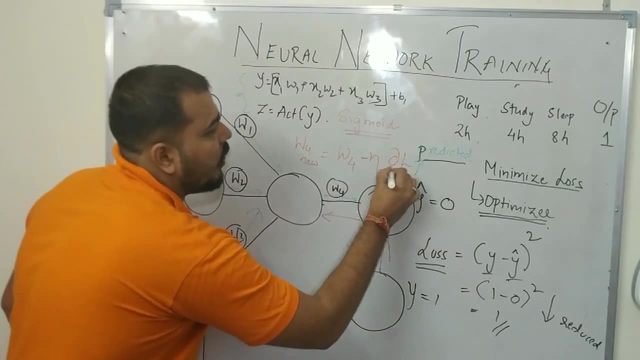 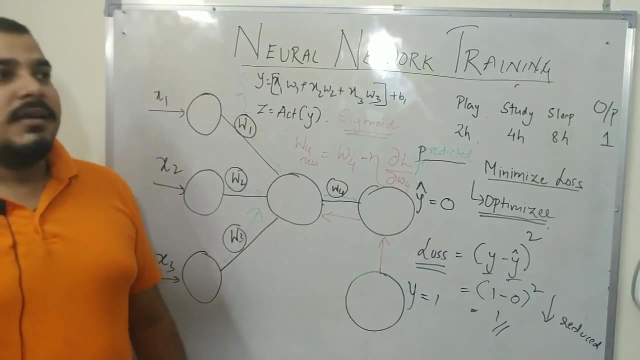 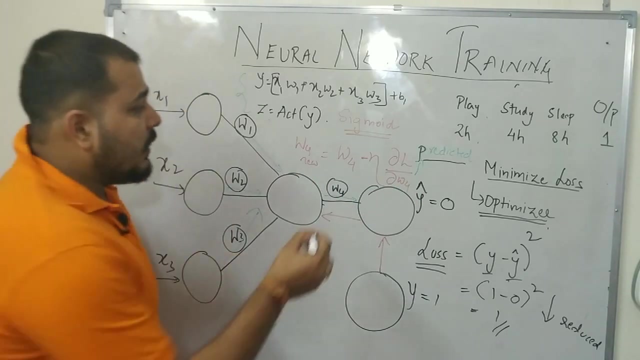 minus. okay, a learning rate, a learning rate which I'll just show it in a small n. Okay, And then I will find out the loss of the loss function, derivative of the loss function with respect to W4.. Right, So here we are actually trying to find out the derivative of loss with respect to W4.. So this W4, whatever derivative we will get along with the. 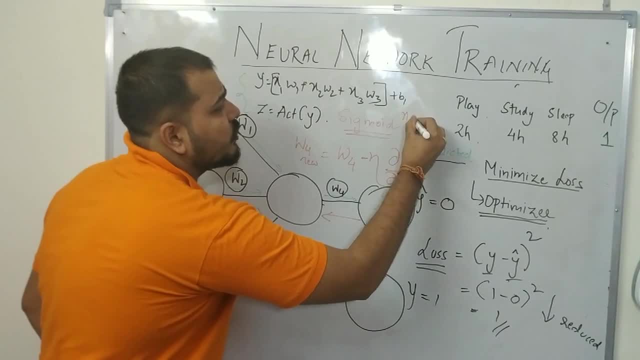 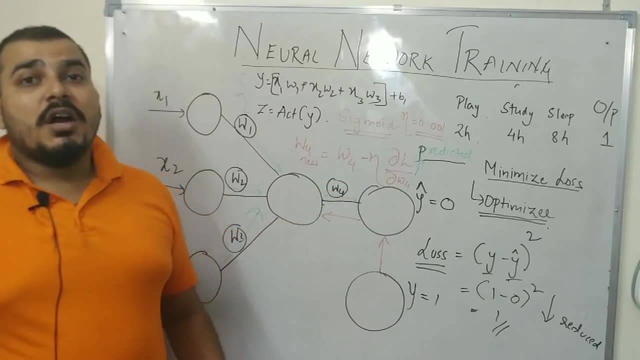 learning rate, which is actually a very small value. learning rate should be a very small value. Suppose I'm considering this as a small value. The reason I'm taking it as a small value? because it will help us, to you know, go to the global minima function in the gradient descent whenever we want to actually achieve that particular point, And that is only possible by this particular optimizer. Suppose if you're considering gradient descent, we'll discuss in the next upcoming classes what are the different kind of optimizers. this weights will get updated in such a way. 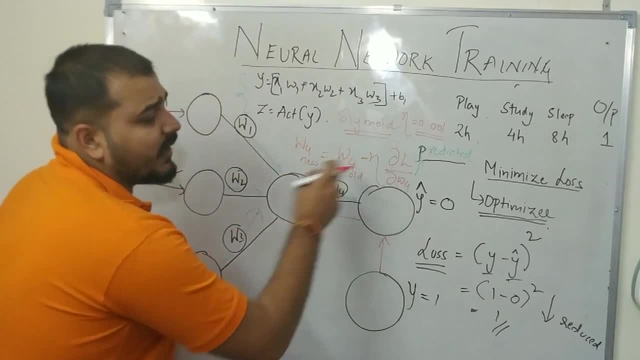 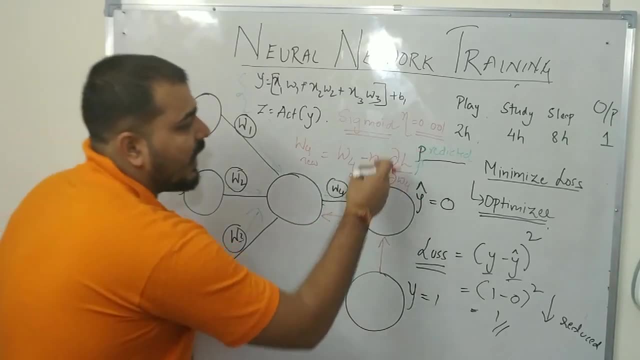 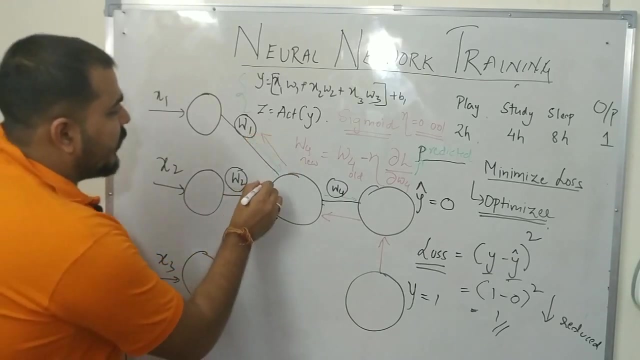 a way that this W4 old value will get subtracted with the learning rate multiplied by the derivative of W4. And the derivative we are calculating is with respect to loss function. So once we calculated this derivative, then we need to update W1. also, We need to update W2.. We need to update. 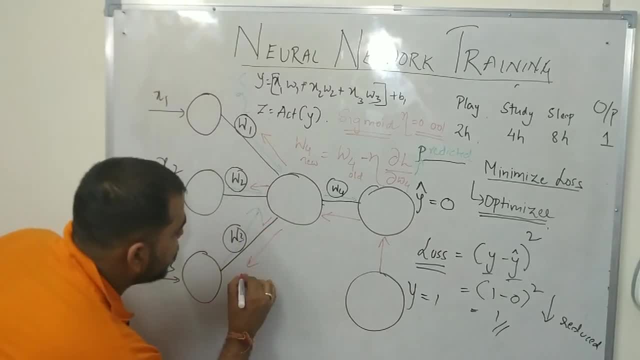 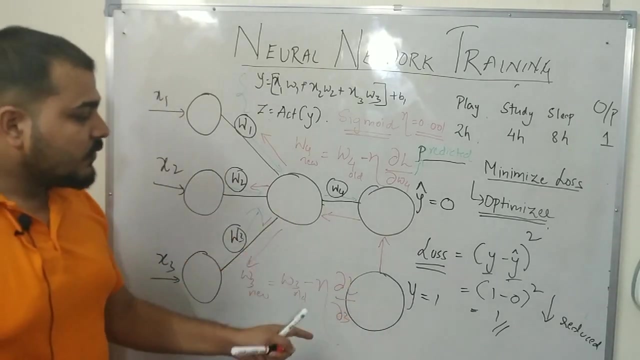 W3. also, In the case of W3, again, how this will be, We will have W3 new value. It will be W3, old value, minus learning rate, minus learning rate with the derivative of D3.. Derivative of loss with respect to D3. So again, we will get this W3 value. Similarly, we will get the derivative of W2, W1. 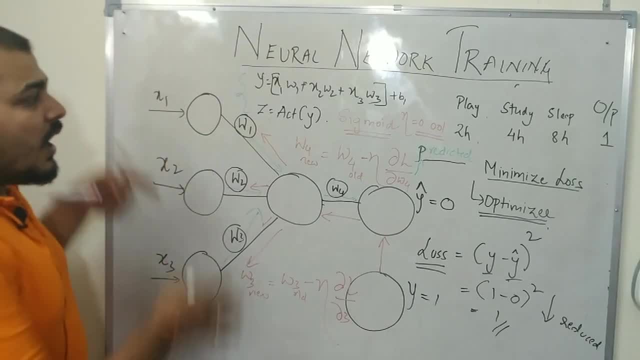 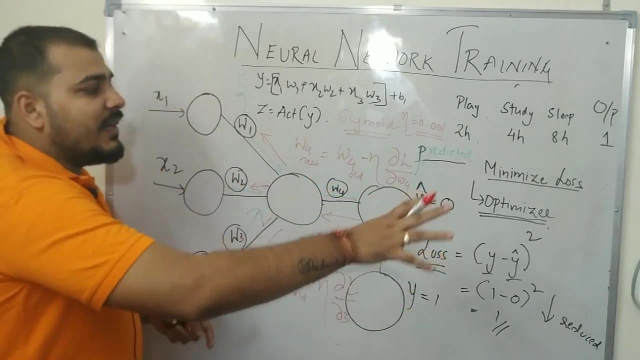 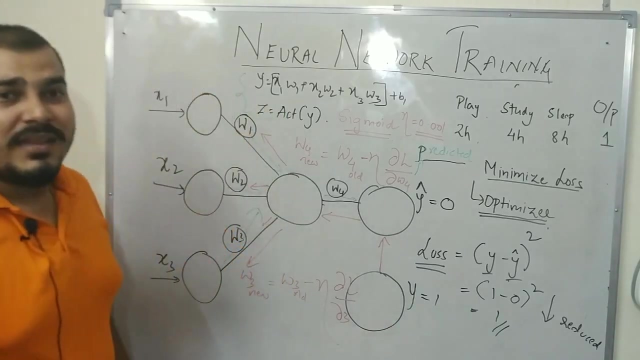 and we will get the updated value. Once we get the updated value again, the front propagation will go ahead Again. the same process will go ahead. It will go unless and until, you know, for some number of epochs, Unless and until this loss value is completely reduced. So once it is reduced, you will be seeing. 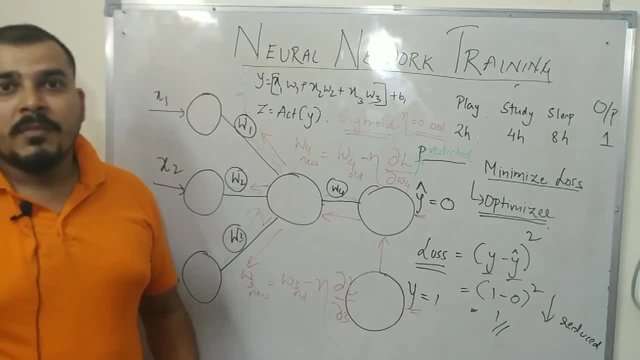 that Y hat and Y will be matching. finally, And this was all about the training, the neural network. There are a lot of problems that basically happens in this is something called as vanishing gradient, you know, exploding gradient, which I will be discussing in the next classes, But just 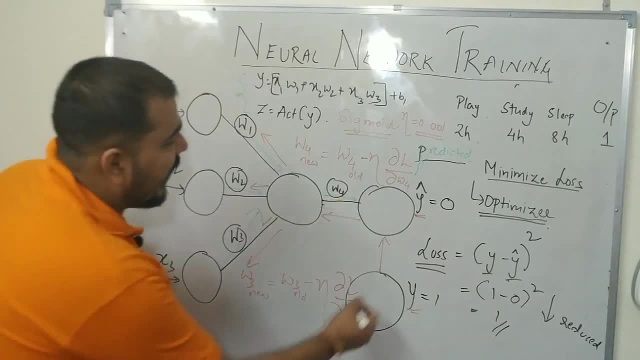 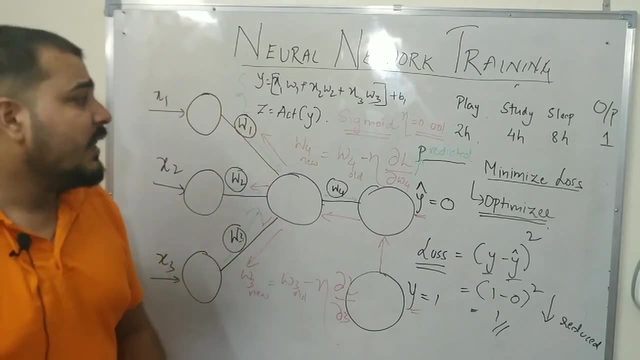 understand that how the normal forward propagation and the backward propagation has happened. The red line that I have drawn is basically my backward propagation, where I am updating the weights right As I go ahead in the green color line. that is basically my forward propagation. 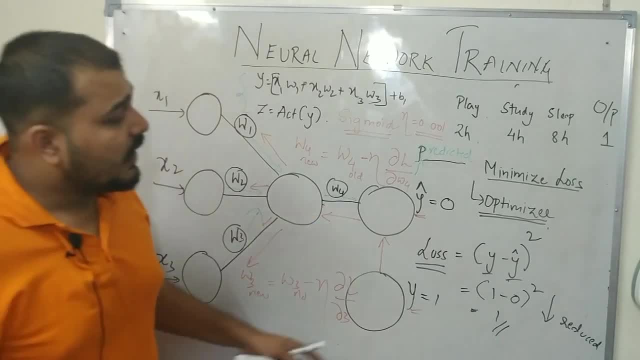 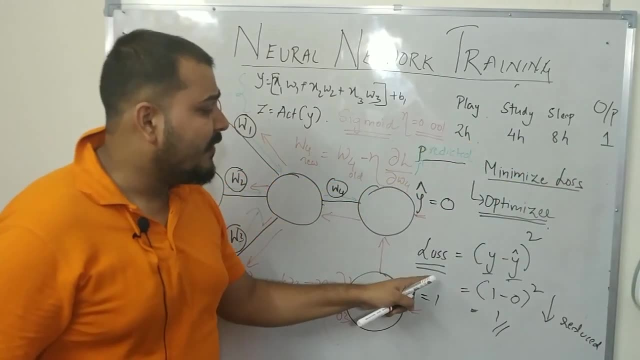 So this process is going to happen for many number of times, unless and until we see our loss function getting reduced completely. Now, since I had a single value, single record over here, so I derived a loss function. But if I have multiple records, at that time I have to define a cost.